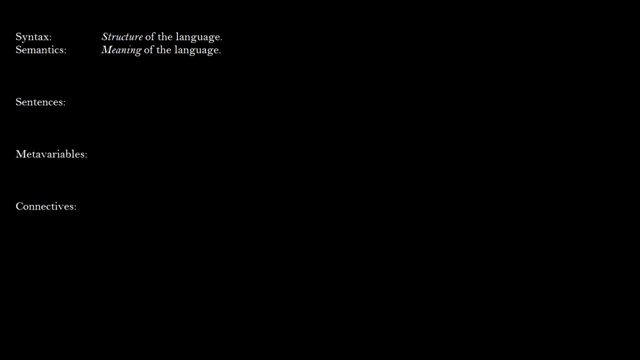 All right. in this video we're going to be taking a look at the syntax of propositional logic, and the syntax is the structure of the language we're going to use. We're going to cover semantics later, which is the meaning of the language, but I prefer to do syntax first and then give. 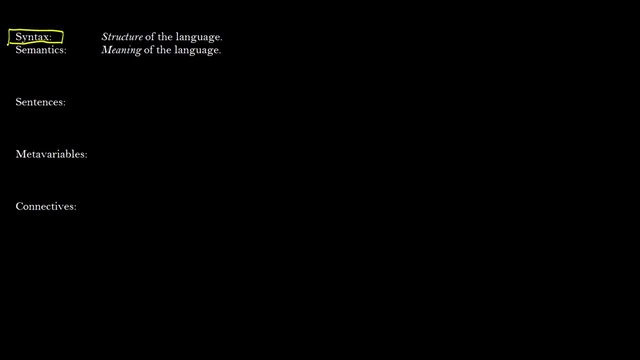 a general idea of what meaning is a little bit after we introduce it. So how are we going to formalize our language? So we're going to have sentences and these are going to be lowercase letters- P, Q, R- and sometimes what we'll do is we'll put little numbers below them. 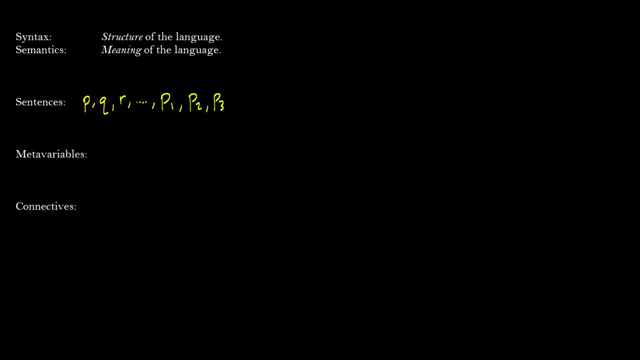 so we'll have P1,, P2, P3, just in case we run out of letters and we want to use the end of the alphabet for this. Sometimes I will use capital letters, and a lot of books use capital letters- P, Q, R and they do the same thing Either way, it doesn't really matter. 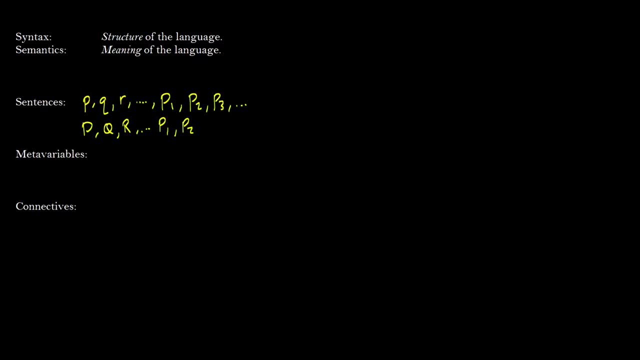 when you get into more advanced logic Sentences are generally just lowercase letters, but I know in the logic book they use capital letters. Our meta variables we're going to use Greek letters: alpha, beta, gamma, delta. and here's the conflict is that some books like the logic book. 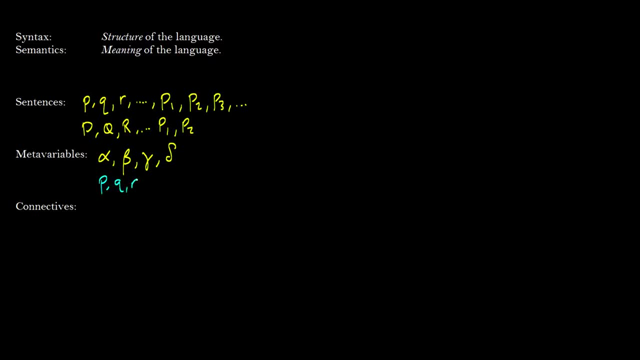 uses lowercase letters As meta variables. I'm going to avoid using lowercase letters as meta variables just because in advanced logic this is the way they do it, with Greek letters as meta variables, and what meta variables are is used for what they call valid forms. So when you don't have a specific argument, 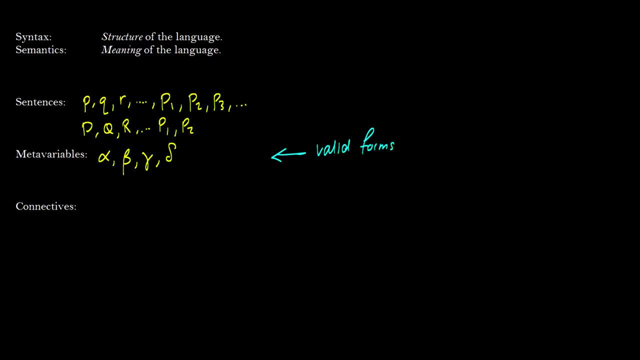 but you just want to show that a form of an argument is valid. you use meta variables. Sentences are generally just lowercase letters and I'm going to avoid using lowercase letters, as sentences are for specific instances of an argument. So if I want to say that I want to talk. 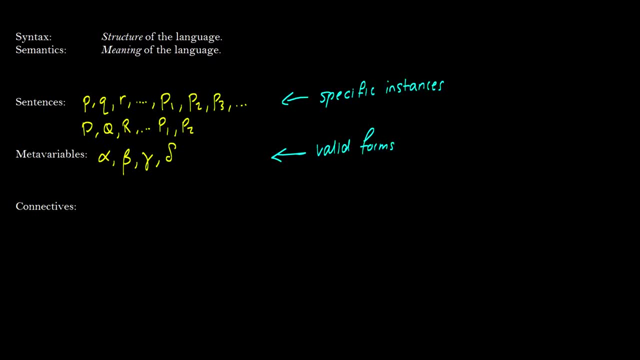 specifically about my trip to a baseball game. I would use sentences for an argument, but if I wanted to use a meta variable, it could be used for any situation, and we're going to see a little bit of this later. We also have connectives in our language, because we need words that connect sentences. 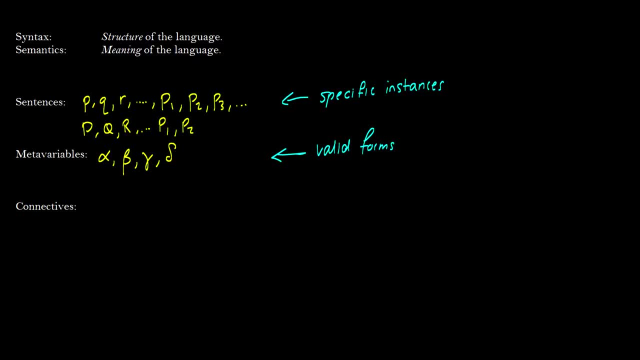 together. So we're going to have: if we have a sentence p, we can also have a sentence not p. so this is not. Some books use a squiggle for p, so use a tilde p. I'm not going to use the tilde because 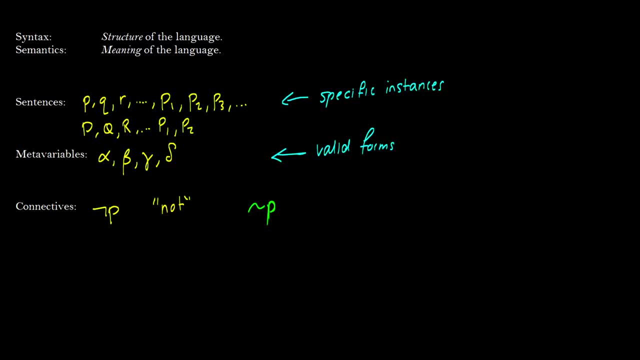 I think it doesn't look as nice. It's good for typing if you don't like to use LaTeX, but it makes things a little bit more difficult, So I'm going to use a tilde p We are going to have and which is called a caret. It's an upside down v. A lot of books will use the. 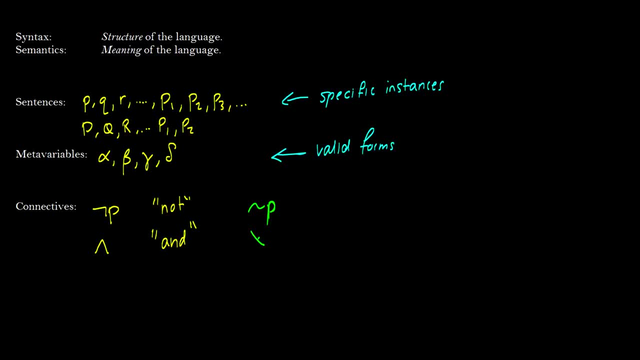 and symbol, the ampersand. You can use that if you want. Again, instructors will vary. There's an or, which is a v, and most people agree with this. Some people use a plus sign in computer science, but that is very rarely seen, And you also might have an ancient textbook that uses a dot for the. 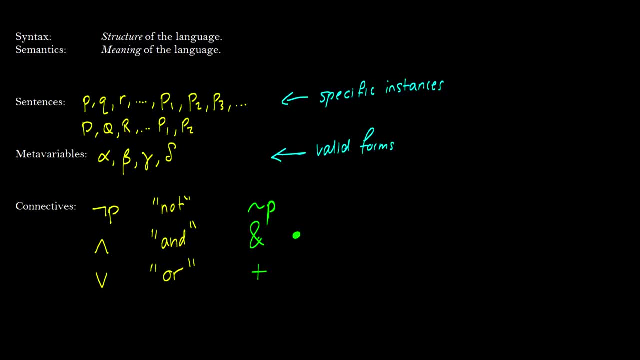 word and That is not commonplace at all. So if your instructor is using a dot or you see a book with the dot, I would suggest not learning the dot, because it's something that is never used and people will give you funny looks. We also have an arrow, which is our if-then arrow. 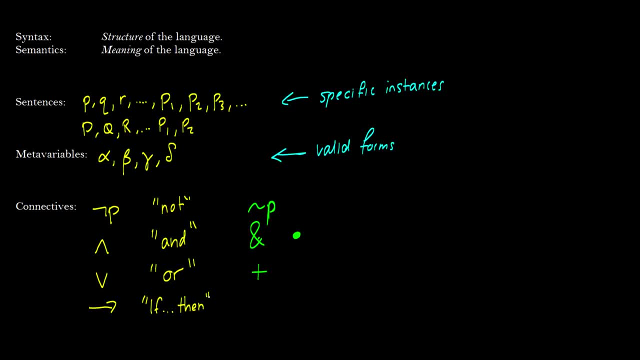 which you might remember from the first video when I did a test with the sentence: if I'm a boy, then I have genitals And some books use this weird horseshoe-like thing And it's perfectly acceptable. but I'm going to tell you why you shouldn't use. 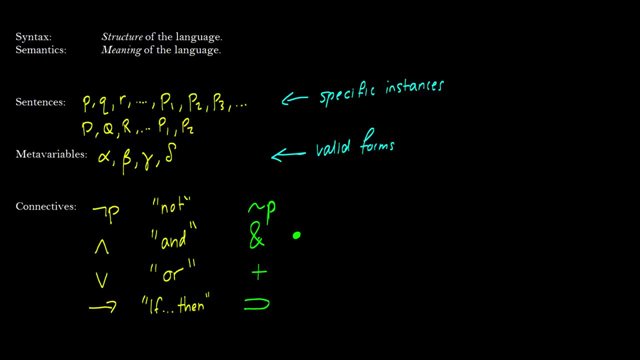 it. You shouldn't use it because this is also the same symbol used for a superset, which is something used in advanced logic, in hypergraphs and other sort of things. So I would avoid that And equivalently have the biconditional, which is a double arrow, which is if and only if. again, you 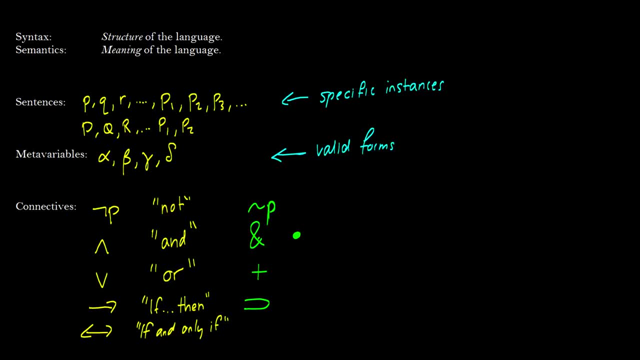 don't. you might not know what all of these mean right now, and that's okay because we'll get to it. sometimes they use the triple bar for equivalents there. so these are our connectors. in the language, we only have these five to connect sentences, so we have a bunch of things here that you know. you kind of. 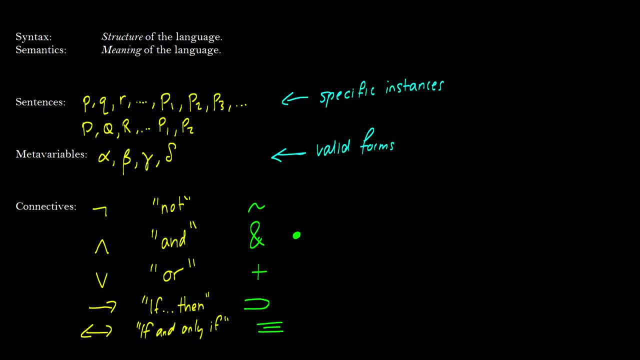 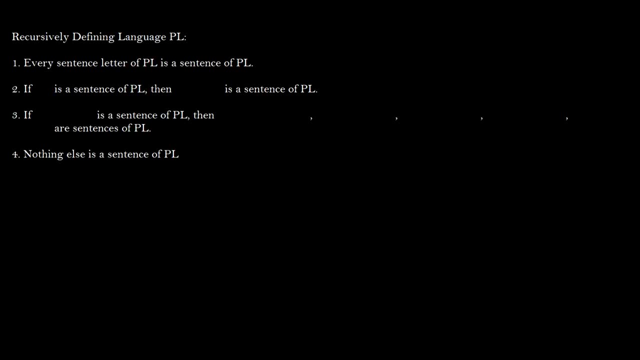 know what they mean, but how do we put them together? well, this is what we're going to do now: we're going to define the language recursively. so what this means is we're going to take a starting point and then we're going to make a couple modifications on the starting point. 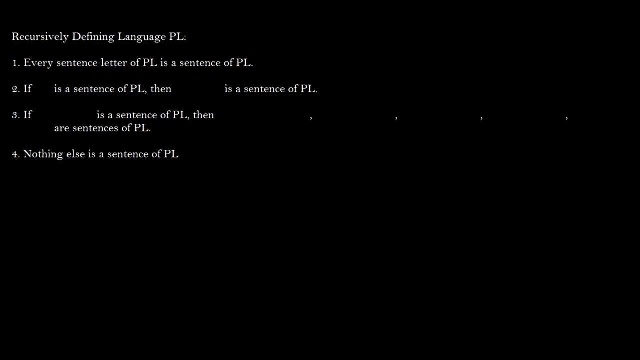 and then everything you can ever make in the language is going to follow from these rules. so we're going to say every sentence letter of PL is a sentence of PL. now this might seem a little bit crazy, but that just means that we can write down P and that is a good sentence in our language, P and if we have P is a. 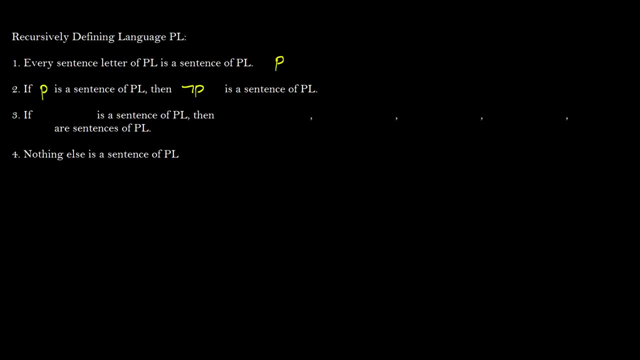 sentence. then we can also say: not, P is a sentence, so that's good. and if we have two sentences- P and Q- you should be in our sentences sentences. then we're going to have some things we can do with this. we can say: P or Q is a sentence, PVQ. we can have P and Q, just P. 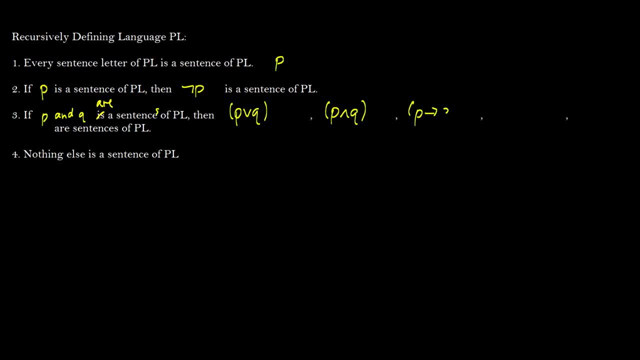 carrot Q. we can have if P, then Q, and we can also have P if and only if Q as sentences, and nothing else is a sentence. in a book. this would normally be listed as conditions 3, 4, 5 and 6, just because they like to break it up. but there's no. 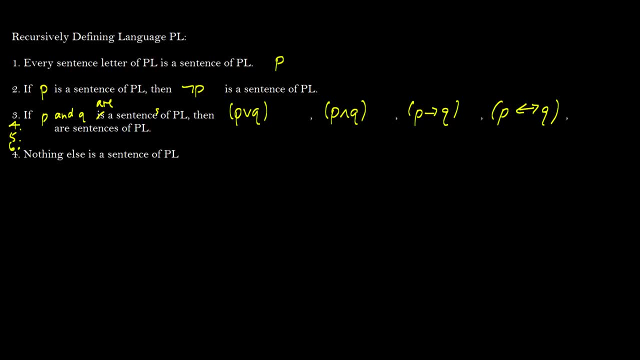 need to, and nothing else is a sentence of PL. so PL is our language, so let's let's have an example here. I want you to tell me if this is a valid sentence in our language. and don't be confused by the letters. this is any general letter. 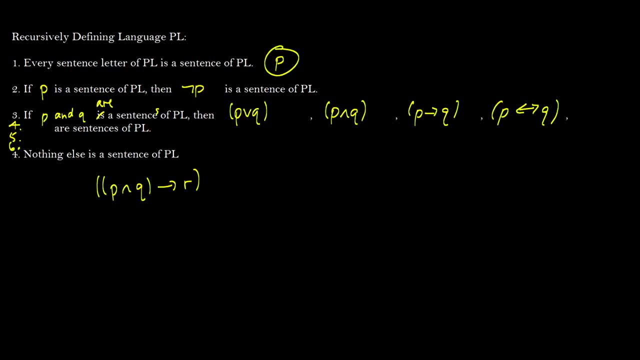 is a sentence, so you can pick any letter you want and it's going to be a sentence. so the answer here is yes, and what I should mention here is that we also have brackets as part of our sentence, as part of our language anyway, and we need the 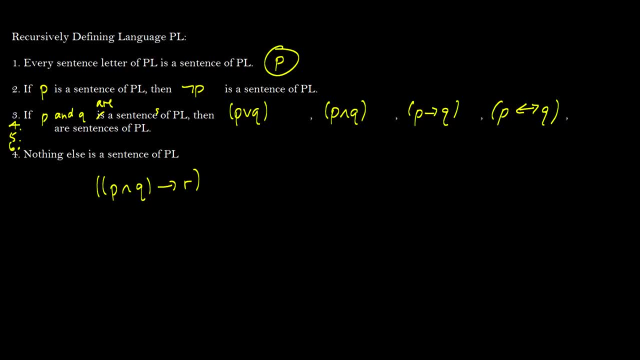 brackets to be, even. if the brackets are not even, then it is not going to be a valid sentence. so it is going to be, because here we have P and Q is a valid sentence, and then we've connected this sentence. you connect to this sentence, right here. 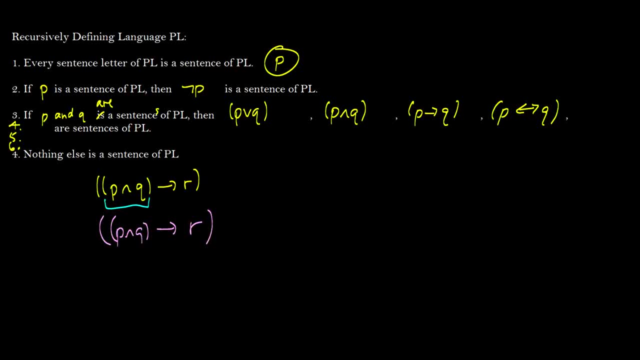 with another sentence are we put brackets around it. so this is good. what would it be good is if we said: okay, what about P and Q are? well, we have no rule that says that we can take a letter and put a rape aside- another letter it needs. 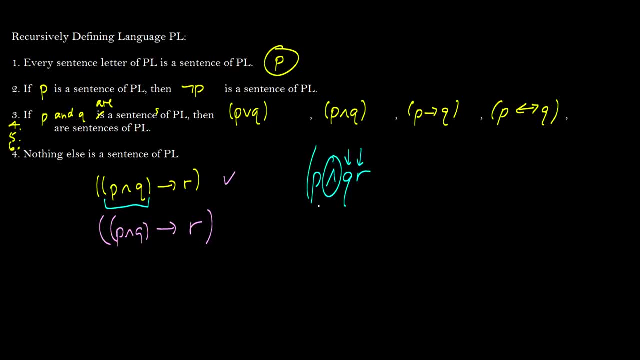 some sort of connected between the two and they also need to be bracketed. and I should mention now moving forward, we are not going to include the outer brackets on our arguments, so just to have P and Q arrow R is also acceptable, because we just assume that there are brackets on the outside. that is not. 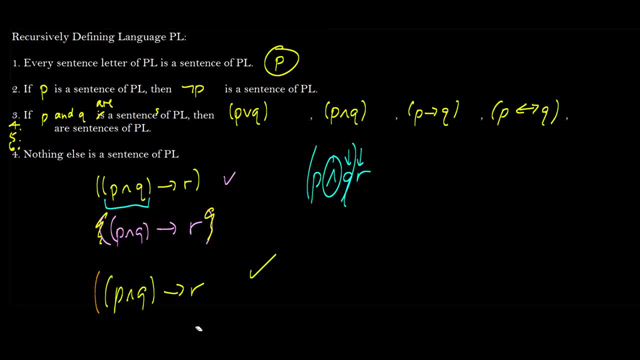 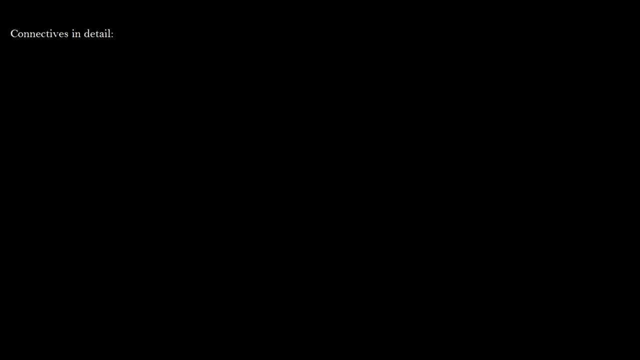 something that you have to explicitly write down. so here's our language, and now we're going to talk about our connectives a little bit. so we have a few, we have and which takes two arguments. we have, or, and which takes two arguments, We have if-then, which takes two arguments, and then we have the. 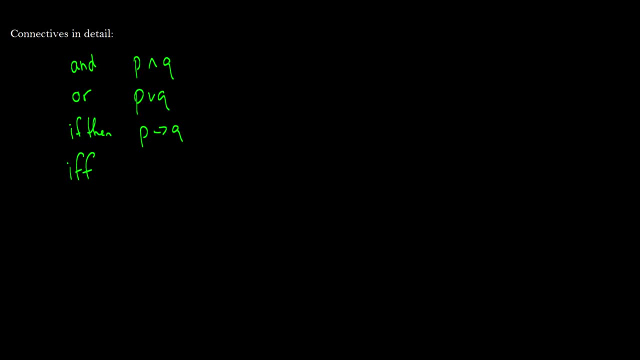 if-and-only-if, which is just if with two f's, and this is p, double arrow q, And these are all binary connectives, and binary connectives means that it connects two things, so it connects p and q, and we also have one unary connective, which just means connecting one thing, which is: 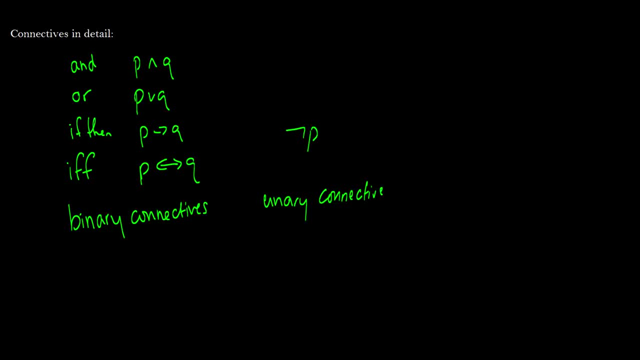 not p and this is not. So now I bet the question is: well, you see words like conjunction and disjunction in books, so we're going to give these sentences a little bit fancier names. So p and q. this is called a conjunction, So we conjoin two together, so it's a conjunction In a Venn diagram. 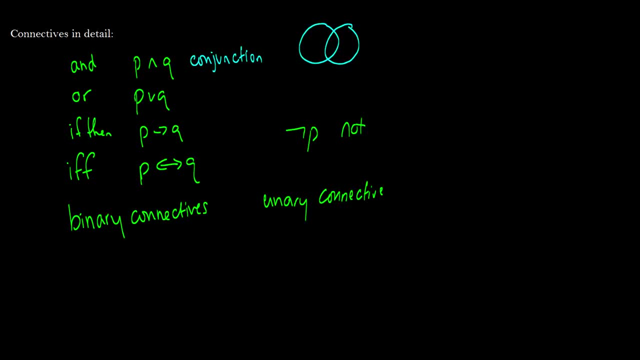 I don't really know if I want to do this, because this isn't set theory, but it's the situations where they're both true, Or it is called a disjunction, and what a disjunction is. let me just move this over to the side. a disjunction is when: